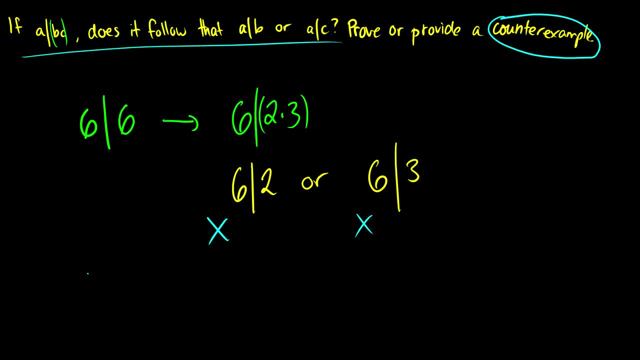 And of course, the easiest way to start is usually with the number one, But if you do ones you get some problems. So you can start with two. You can say two divides two, This is two divides two Times one, And you get some problems there. So, picking these simple counterexamples to test, 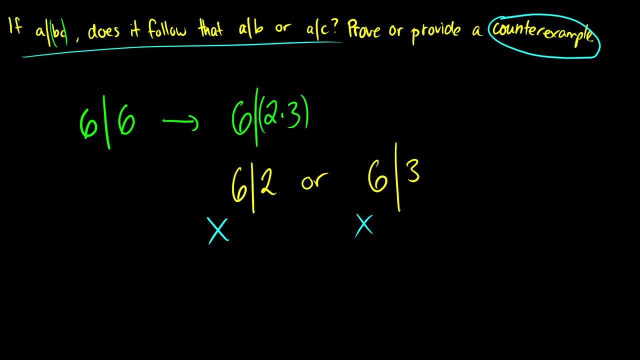 is usually a nice choice to start a disproof. Okay. second question: If n is a positive integer and n is odd, we want to prove that four divides n squared minus one. So we have: n is odd and n is a positive integer. So we have: n is odd And n is a positive integer. So we have: n is odd And n is a positive integer. 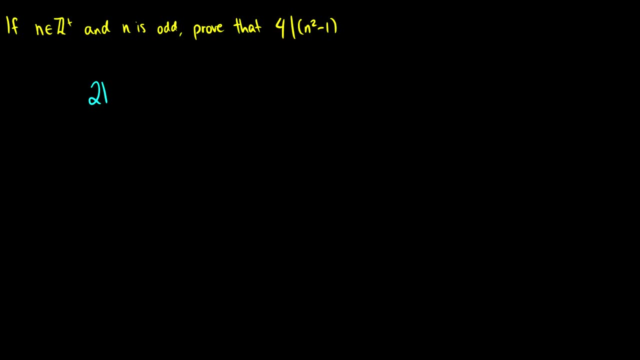 This means that we have 2k plus one, And this is what n is equal to. So we want to prove that four divides n squared minus one. So let's take n squared minus one. So n squared minus one is going to be 2k plus one squared minus one, which is 4k squared plus 4k. 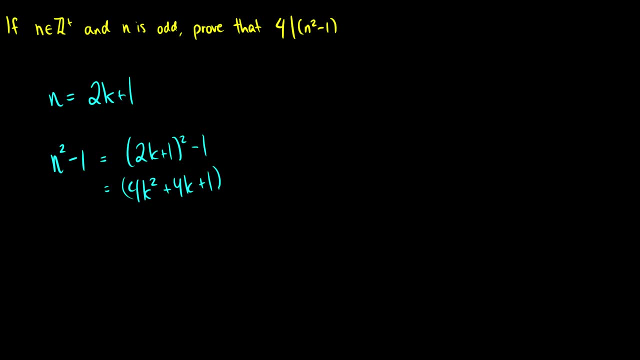 plus one, all minus one. So we're left with 4k squared plus 4k, And then we can factor out this four, which is k squared plus k, And there we have it: n squared minus one is divisible by 4.. So relatively simple proof. Now we can extend on this a little bit, So let's use the 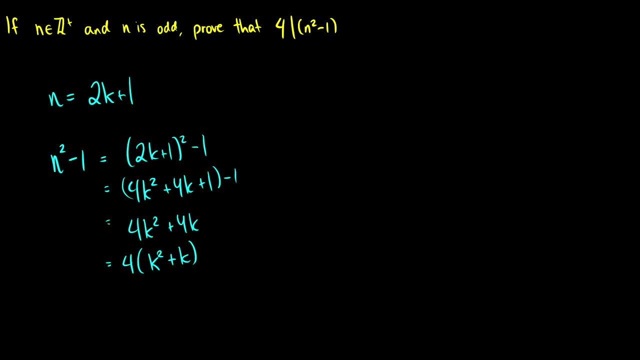 Then we can extend on this a little bit. so let's use the relatively simple proof. now we can extend on this a little bit. So let's use the little bit. now we can extend on this a little bit. so let's use the: or by four planet, Or maybe it's more than, Yeah, four Planet, Or maybe it's over. So let's use the. 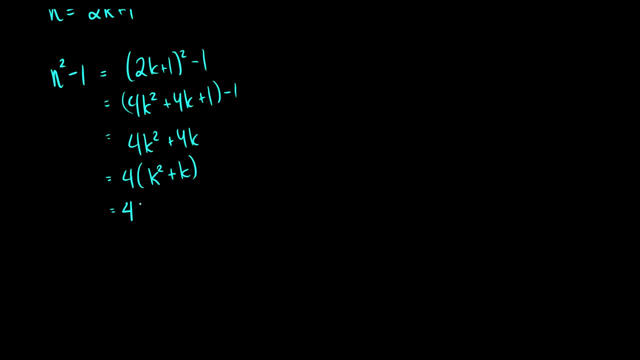 let's fully factor this. So we have 4k times k plus 1.. Now can you take this? and yet can you prove that 8 divides n squared minus 1? So 8 divides n squared minus 1.. So let's think about: 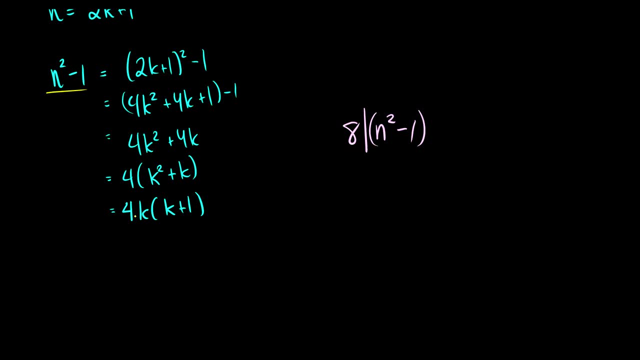 this one. We have n squared minus 1, we can factor out this 4k, So really we can rewrite this either way. So we can say: this is equal to 4k times k plus 1, or this is equal to 4 times k plus 1.